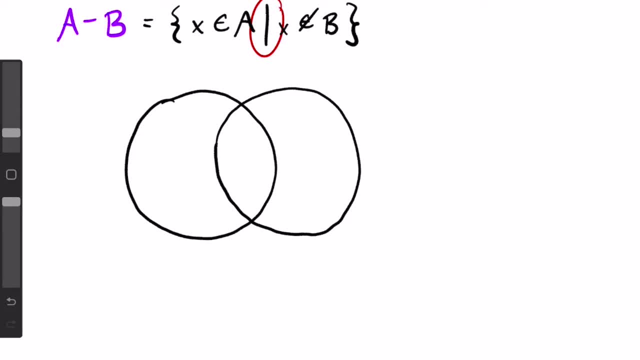 so that's mainly what I'm going to use in this video and in the example problems which are linked in the description below. For a brief refresher, a Venn diagram is a sort of Olympic ring situation where each circle is a different set. So let's say this left circle is A and this 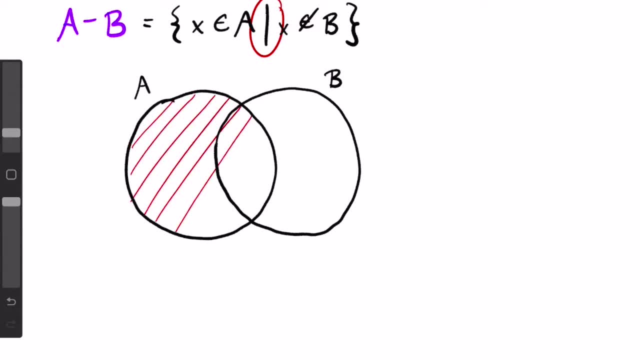 right circle is B, Anything inside the left circle is in the set A and anything inside the right circle is in the set B. So anything in this middle part then would be in both A and B or in A intersect B. Using the Venn diagram, A minus B would be the set of everything in A but not in B. 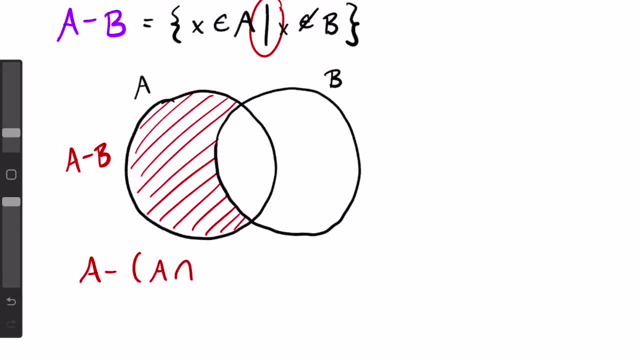 Another way to say this is A minus B. A intersect B. This might seem redundant- After all, it's longer than A minus B, so why would you want to use it? But it is what we actually mean when we say A minus B, and it can sometimes be. 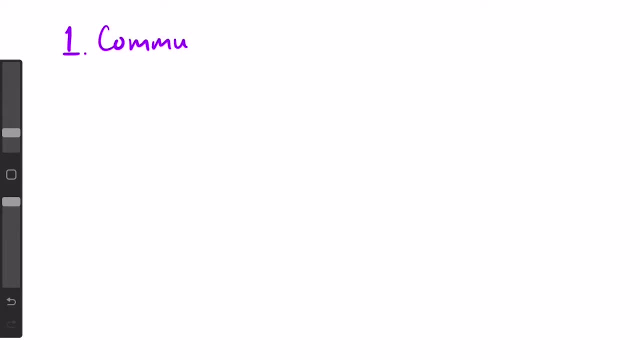 useful for proofs. Now for some algebra. The first property is the commutative property, and it works exactly the same as in regular algebra. It states that A union B equals B union A and A intersect B equals B intersect A, And that makes sense, right? The set of 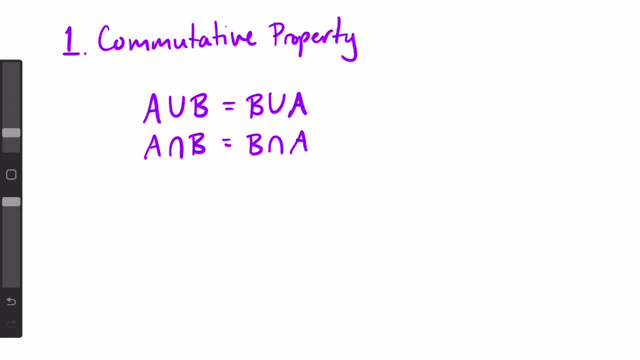 elements in A and B is the same, no matter what order A or B are in. The second property is the associative property, which states that A union B- union C is equal to A union B- union C And same thing for intersection. Note that this does not mean A union B. 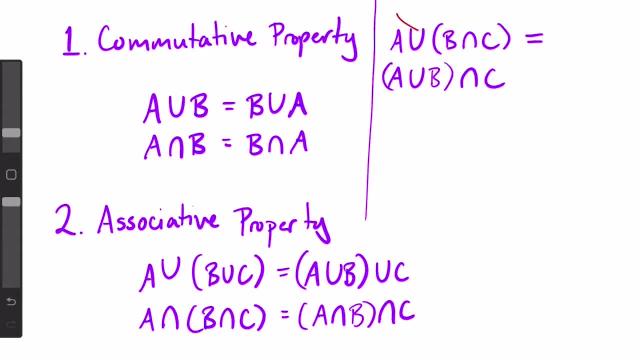 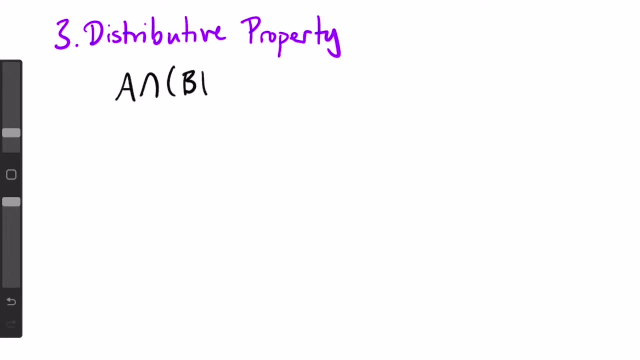 intersects C is equal to A union B intersects C Or the other way around. you can't re-associate sets across different types of operations. that is, union and union intersection in the same expression. the third property is a distributive property, which states that a intersect b union c equals a intersect b union a intersect c and the other way around. 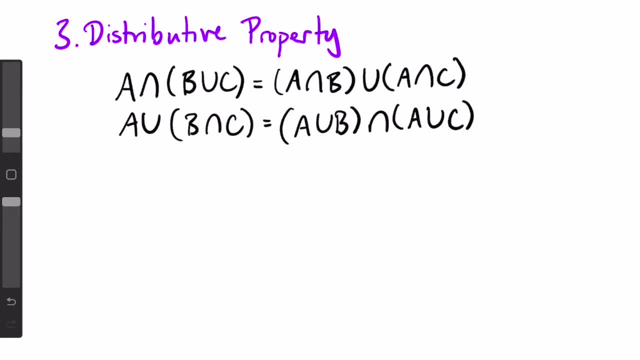 again. it works exactly like it does in regular algebra. you can think of the operation outside the parentheses as a multiplication symbol and the operation inside the parentheses as an addition symbol. a times b plus c equals a times b plus a times c. we can quickly show this is true using 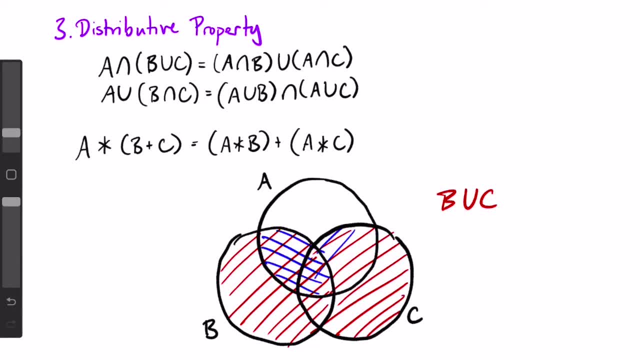 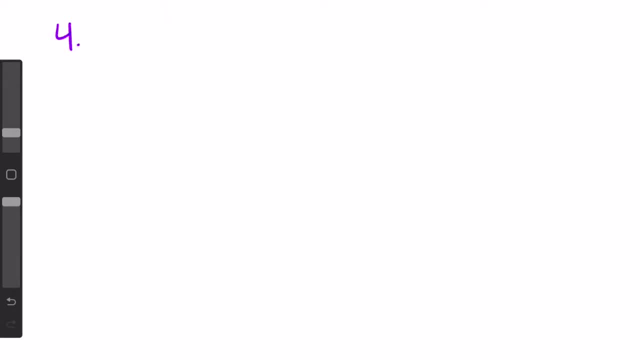 a venn diagram. b union c is this area and a intersect b union c is this part. that's the same as a intersect b union a intersect c. the fourth property is known as de morgan's law. it might be familiar to you if you do computer science or if you know anything about mathematical. 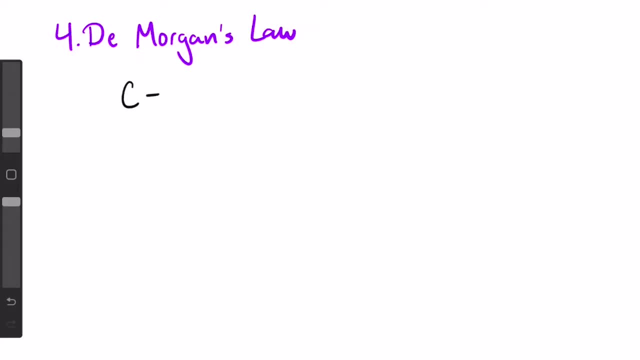 logic. de morgan's law states that c minus a union b equals c minus a union b equals c minus a union, b minus a intersect c minus b. and c minus a intersect b equals c minus a union c minus b. basically, you distribute the minus within the parentheses and then you flip the operation being: 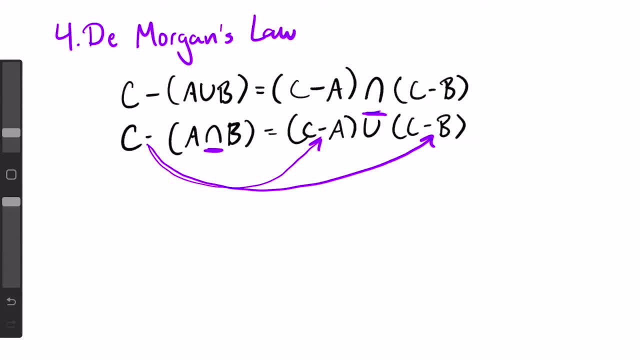 used. a visualization of this is in the example problem, so make sure to check those out at the link in the description. and the very last property is just some identities involving the empty set. these are: a union empty set equals a. a intersect empty set equals the empty set and a intersect c minus a is the empty set. nothing is in the empty set, so the set. 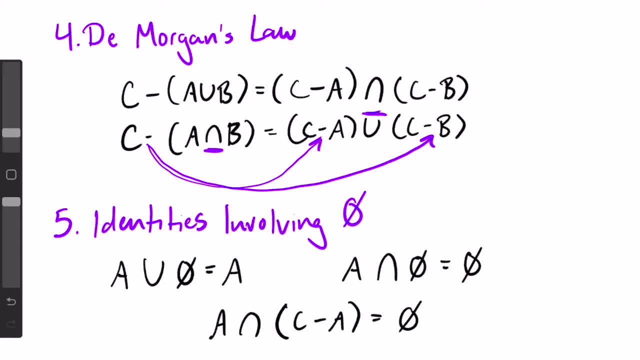 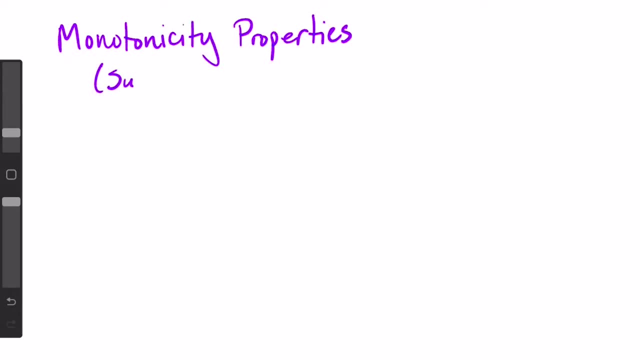 of everything either in a or the empty set is just a. the set of everything in both a and the empty set is nothing, and the set of everything both in a and in the set c, not in a, is also nothing. the next five properties are called the monotonicity properties. that's a very long word, so i'm just 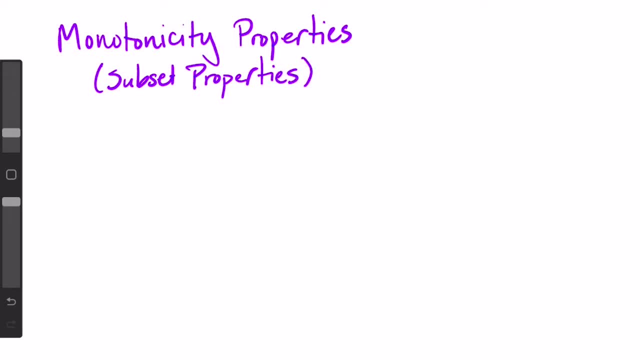 going to call them the subset properties because they're all conclusions that come from. a is the subset of b. these don't have their own names or anything, so i'm going to try to go through them pretty quickly. first is for all sets a, b and c: if a is a subset of b, then a union c is a subset. 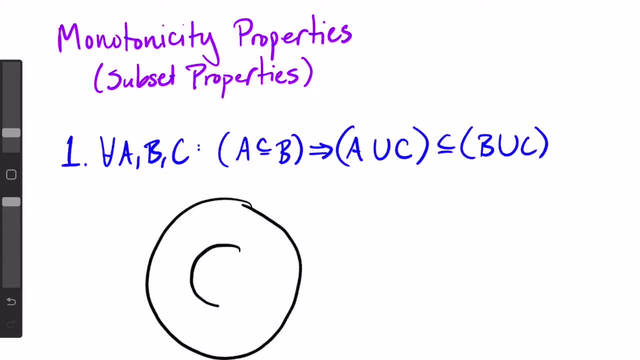 of b. union c. in venn diagram form we can draw a and b where a is fully inside of b because it's a subset. then we can draw c over here. a union c is a subset of b. union c next for all: a, b and c if a. 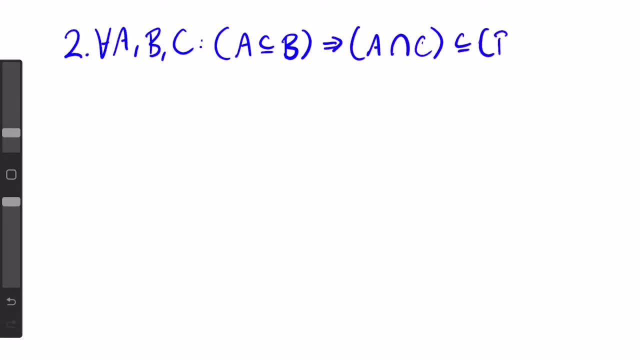 is a subset of b, then a intersect c is a subset of b. where a is fully inside of c, then a intersect c is a��면 c subset of B- intersect C. This is essentially just the first property, just with intersection instead of union. In the Venn diagram that would look like this And you can see that the part of C 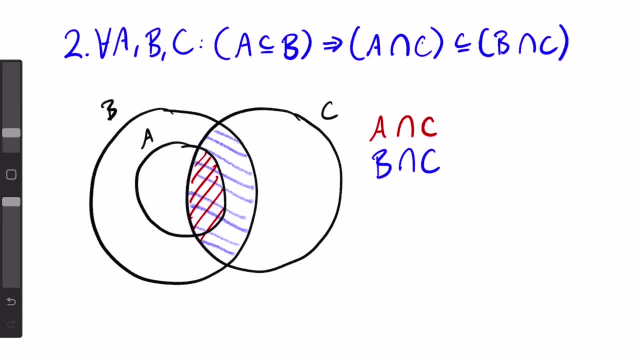 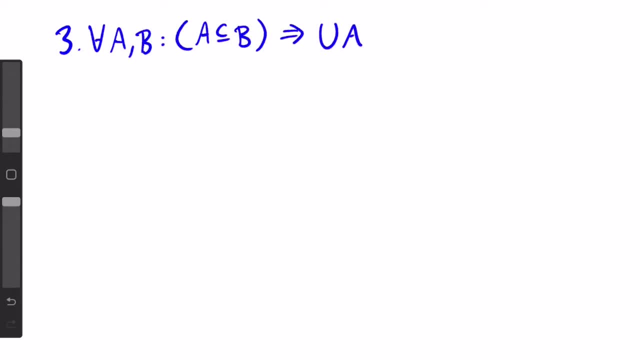 that is intersecting with A is just inside the part that intersects with B, because A is inside of B. Next is for all A and B. if A is a subset of B, then union A is a subset of union B. For a refresher on big union, click on the card to watch lesson 2.. Let's visualize this with another. 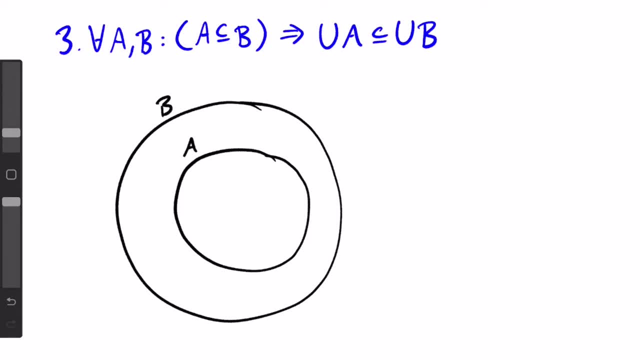 Venn diagram. We have A inside B and this time A and B are sets of sets, So we can draw some partitions representing the sets that make up A and B. These partitions can intersect with each other, just as sets inside the bigger sets A and B can share elements. So A is the set of this set. 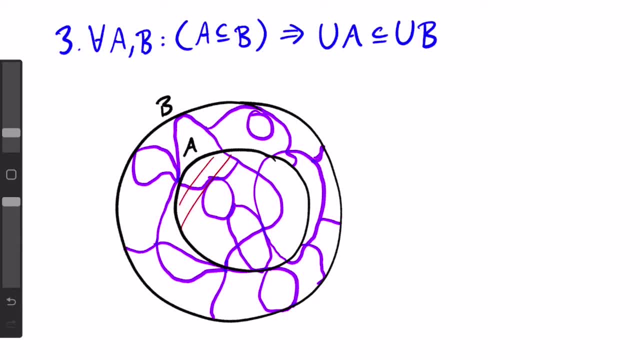 this set, this set, etc. Given these partitions, union A is just this entire space inside the A circle And union B is just this entire space inside the B circle. So we can see how, if all the members of A are also members of B, union A would be a subset of union B. The fourth subset, property, is for all. 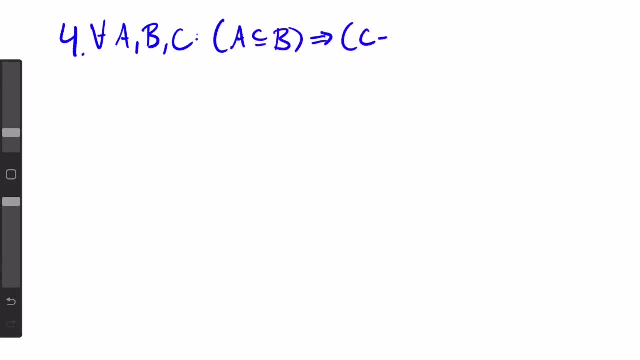 A, B and C. if A is a subset of B, then C minus B is a subset of C minus A. Drawing it out, here's C minus B and here's C minus A- We can see that when we minus B, we're just taking away. 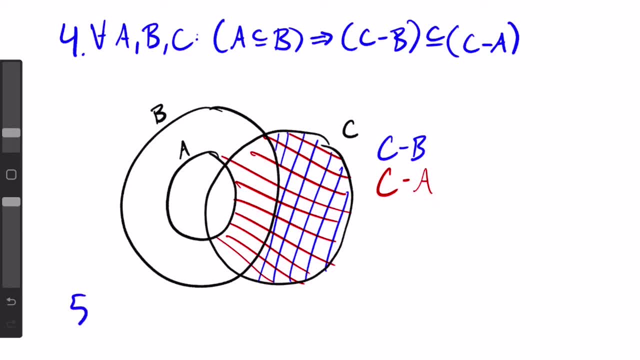 the part that's minused for A, plus a little bit more. The last subset property is for all non-empty A and B. if A is a subset of B, then the intersection of A is a subset of the intersection of B. I'm not going to go through this one now, but a proof of it. 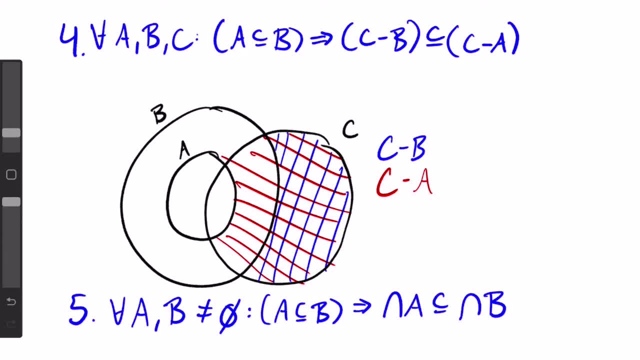 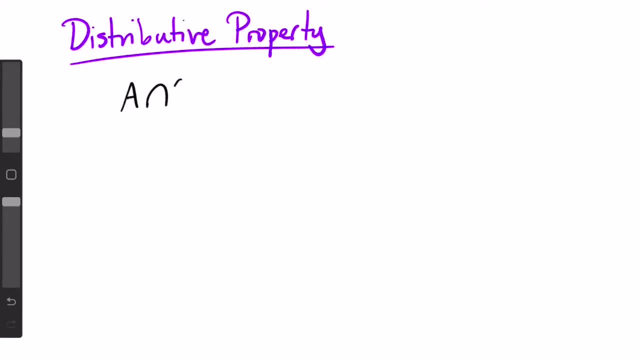 is in the example problems which are linked in the description. The last thing to do is generalize some of these laws. You'll recall from part one of this lesson: the distributive property A intersect B- union C equals A intersect B, union A intersect C And the other version of this. 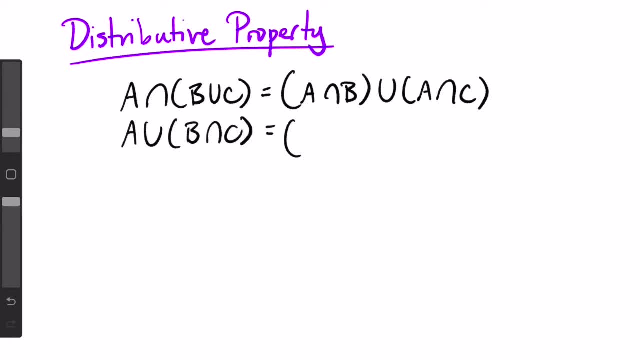 with union is A union B intersect C equals A union B intersect A union C. We can generalize this property from B union C to union S. In the example above, S would be equal to the set of B and C, but it could contain any number of sets that we want to distribute A onto, So the property. 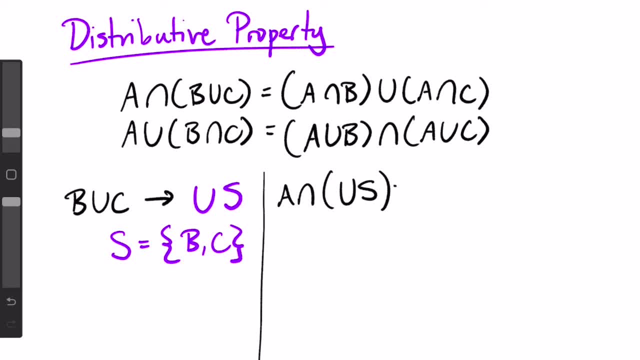 above would become A intersect union S is equal to union of the set of all A intersect B, such that B is in S. remembering that the line means such that And the union version would be A union intersection S equals intersection of the set of all A union B such that B is in S. 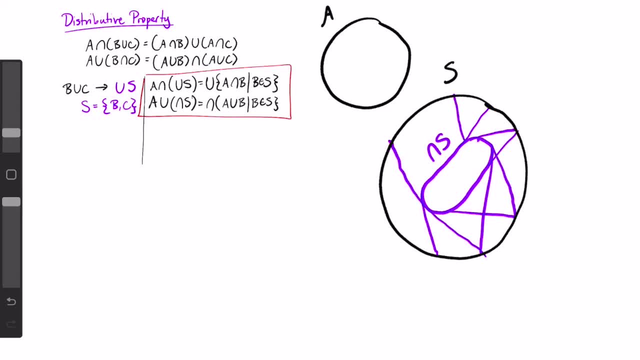 Let's look at the second equation for a sec. What this means is that the set of everything, either in A or in some set in S, is the same as what you get when you union A with every individual set in S, and then you take the intersection of all those unions. 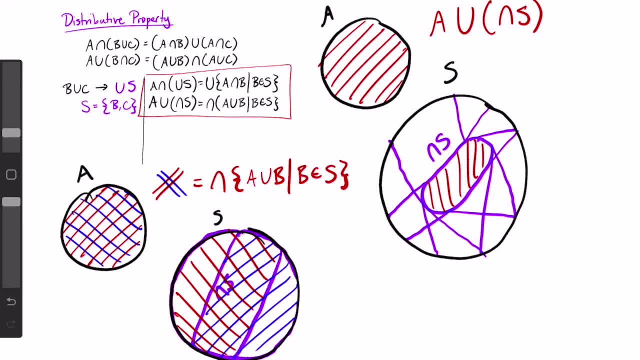 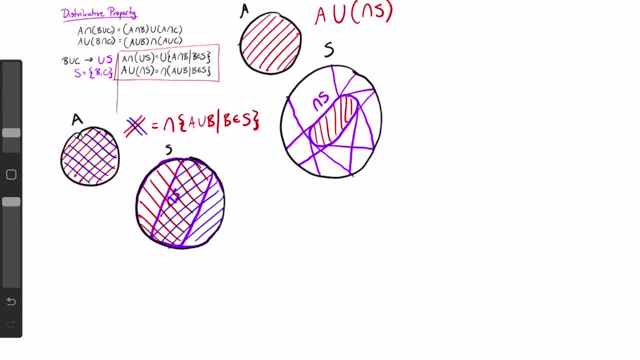 Now that may or may not have clarified anything at all, but the important thing to know here is that this is just an extended version of the normal distributive property and it works exactly the same way. An easier way to think of it may be: A intersect, B union, C union, D union, everything else. 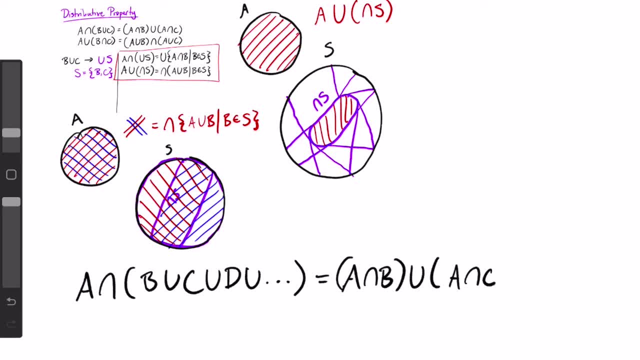 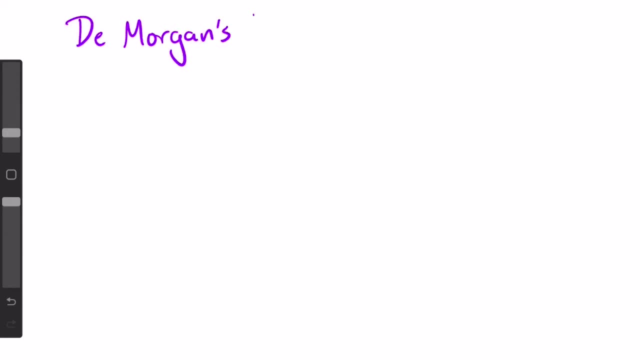 equals A intersect B union, A intersect C union, A intersect D union, etc. etc. where S in the previous example would be the set containing B, C, D, E, etc. The other law we want to generalize is De Morgan's law, To recap from: 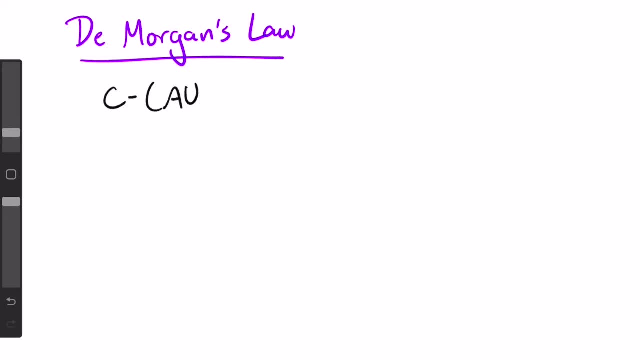 part 1, De Morgan's law states that C minus A union B equals C minus A. intersect C minus B, and C minus A intersect B equals C minus A. union C minus B. In a general format we would write: C minus union S is equal to the intersection of all sets C minus A, such that A is in S and C minus A is in B. 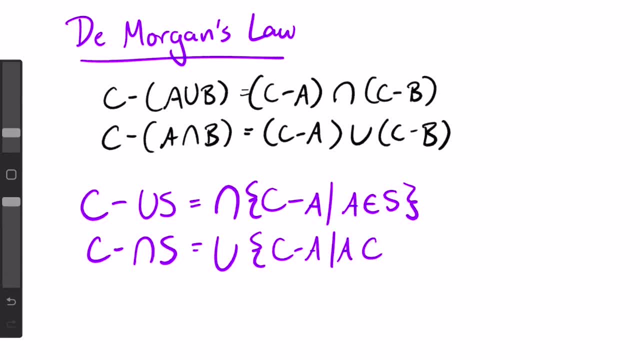 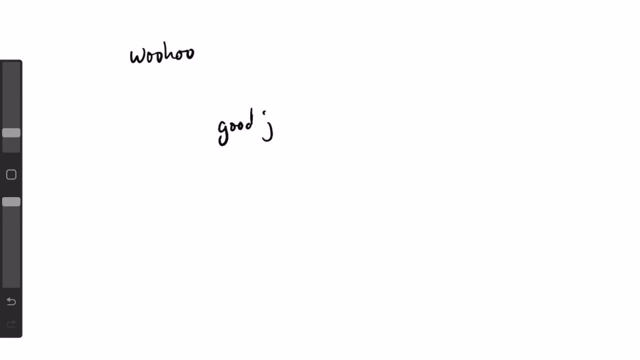 This is the exact same situation as a distributive property, where we just rewrite A union B, union C, etc as union S and the same with intersection. And that concludes the third video of this video series about set theories. I hope you enjoyed it. let me know what you think and if there's 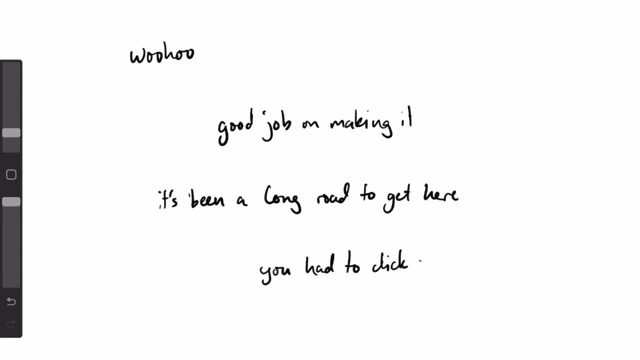 anything that would make it better. Also, make sure to check out the example problems in the description. Thanks for watching. see you next week. Subtitles by Subtitle Workshop.